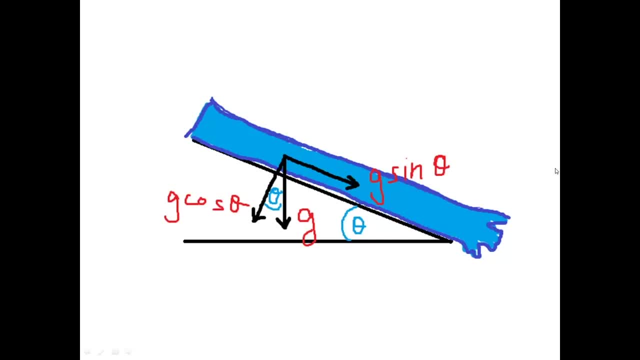 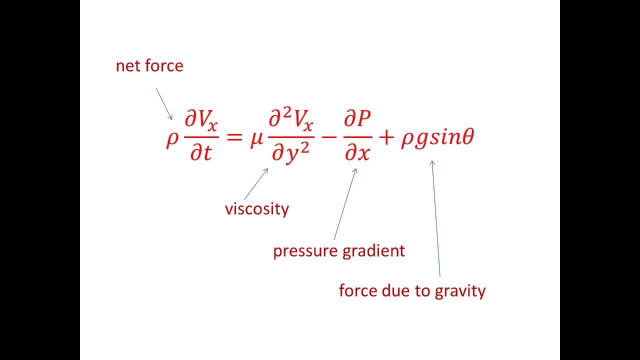 sine theta. We now have an equation that looks much easier than the general form. As you can see, this is just a restatement of Newton's second law. with the viscosity term included On the left side of this equation, you get the net force acting on a unit volume. 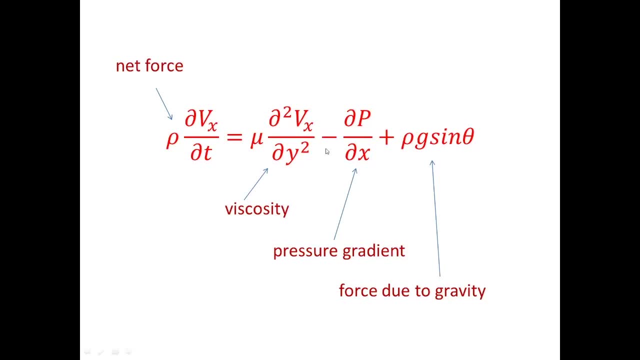 of the fluid. The three terms on the right side of the equation, which are governed by the viscosity, the pressure gradient and the force due to gravity, will be the force due to gravity. Together give the net force acting on a unit volume. 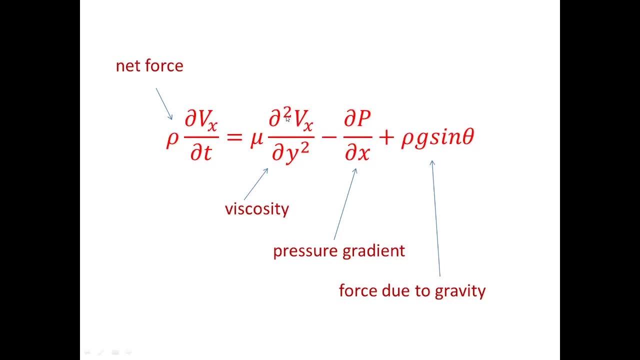 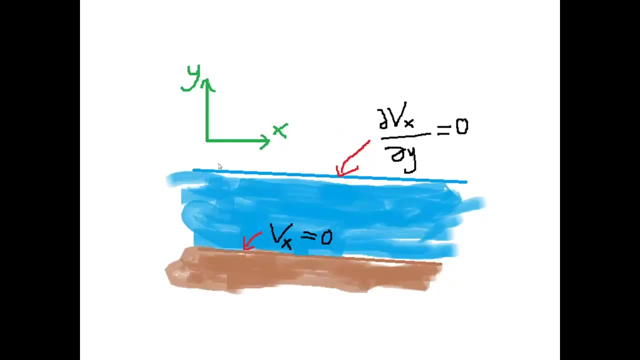 As you can see from this term here, this is a second order differential equation. To solve this, we will have to impose two boundary conditions For the river problem. we will consider the velocity at the bottom of the river to be zero. This is true because the 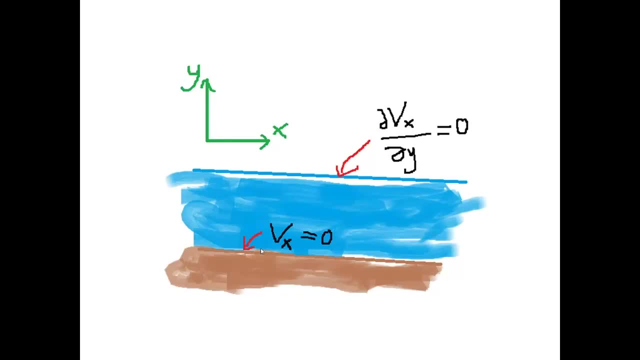 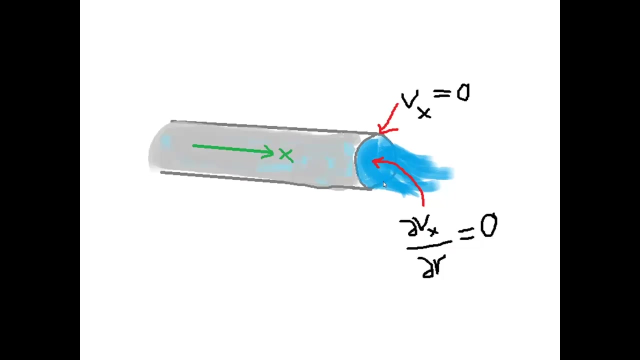 river bed imposes resistance to the fluid layer just above it, preventing its motion, The velocity of the river reaches a maximum towards the top of the river. So we get the condition that dvx over dy equals zero at the top. For the pipe problem, using the same argument, the velocity at the rim of the pipe is zero. 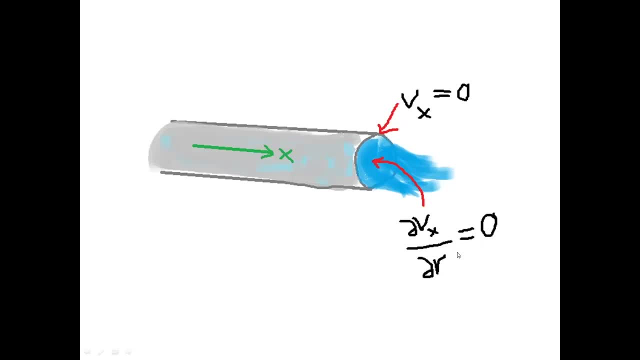 and at the center of the pipe, dvx over dr equals zero, where r, in this case, is the distance from the center of the pipe to the point we are looking at. Now that we have our equation, let's look at it in a different way. For example, let's: 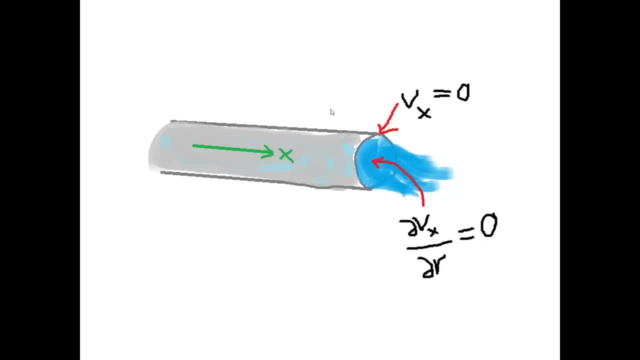 take our differential equation in one dimension and the two boundary conditions needed to solve it, There is nothing left to do but to solve it. We can do this using Mathematica. I was able to solve this equation using Mathematica. In the pipe, the velocity at a distance r. 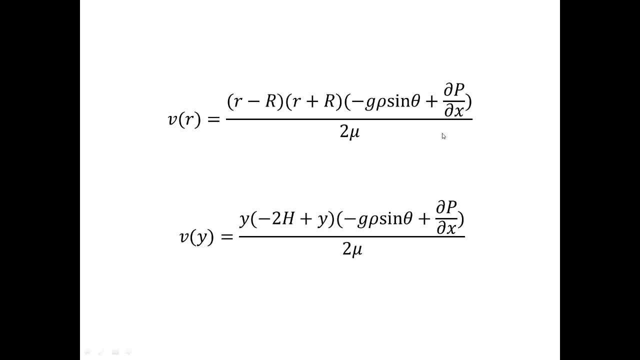 from the center is given by this formula, and in the river, the velocity at a height y from the river bed is given by this formula. If we want to calculate the average velocity inside the pipe or inside the river, all you have to do is add up each individual velocity at all possible radii or heights you can think. 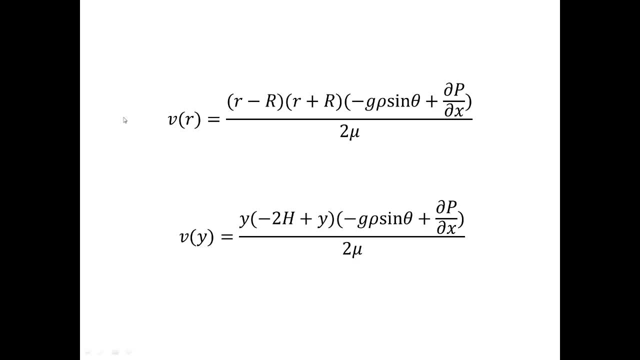 of and then divide that sum by the area that you added it over. It's just integrating and dividing. Mathematica gave me this result. You can see that the average velocity of the fluid in a pipe and in a river increases if you increase the density of the fluid or 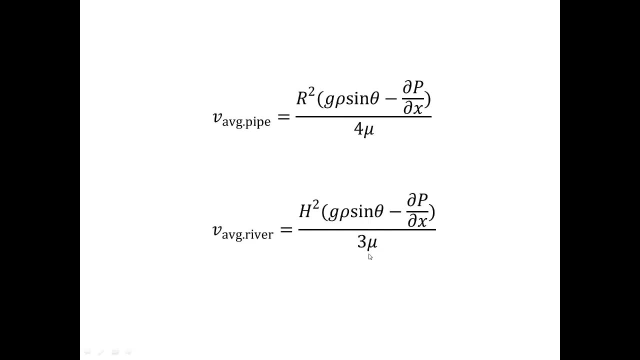 if you increase the inclination of the pipe or the slope of the river to the horizontal. Also, if you increase the negative pressure gradient, the velocity increases. A lower viscosity of the fluid also increases the average velocity. This is all intuitive, but wouldn't it be cool if we could actually model how the velocity profile looks like inside? 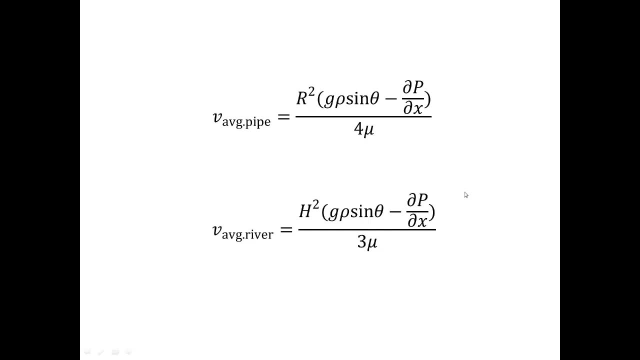 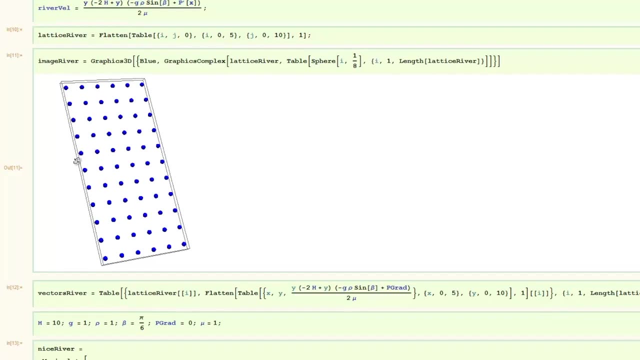 a pipe and inside a river. I'll do this using Mathematica. I will start with the river problem First. I will create a grid of coordinates and for each coordinate on this grid I will assign a vector. This vector will correspond to the velocity. at that point We know how this velocity 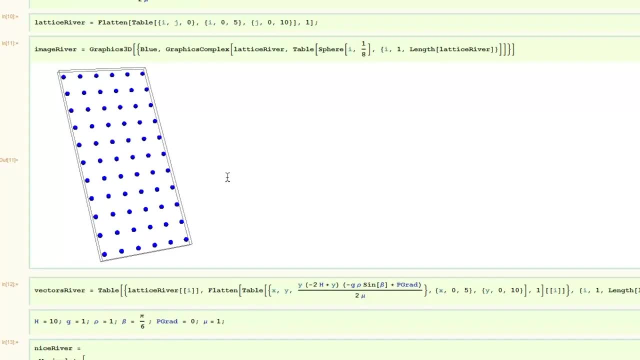 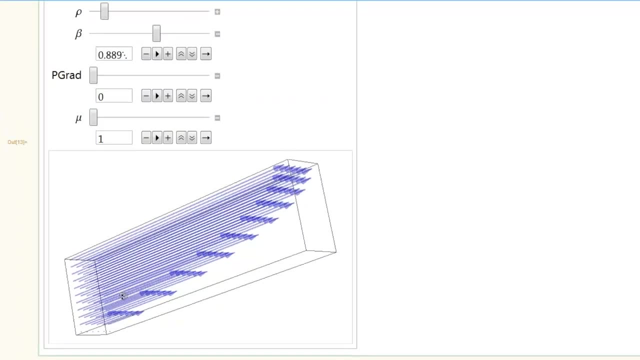 looks like because we solved the differential equation for velocity. Once we have vectors for each of these points, you'll get a picture that looks like this: As you can see, at the bottom of the river, where y equals 0, you have 0 velocity. As you increase y, the velocity. 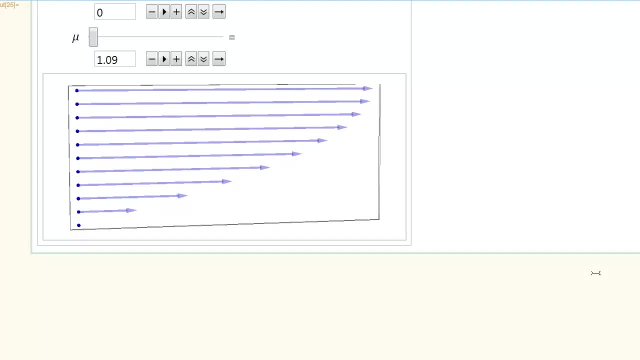 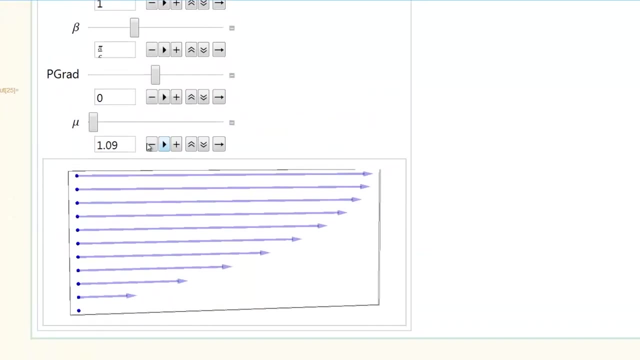 increases. Let's look at just one slice of the previous image. We'll see what happens when you change parameters. When you change mu, the average velocity decreases. Think of these dark blue dots as fixed. These are the reference frame. With higher mu you have lower velocities. 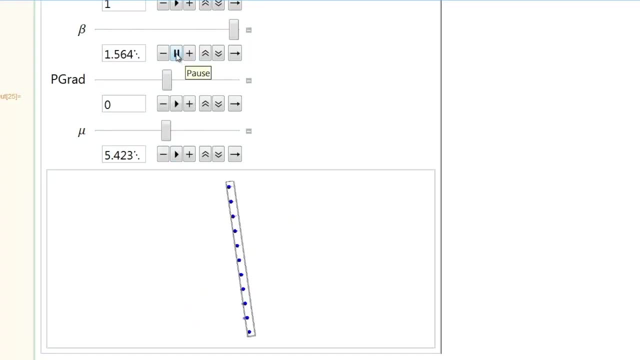 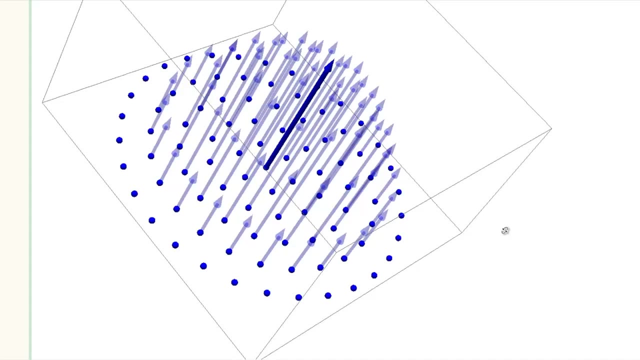 You can do the same for other parameters. I used a similar method to calculate the velocity of the river, For example. let's say the river is a circular grid. I used a similar method to model the velocity profile inside a pipe. I first created a circular grid and then I assigned each point on the grid a vector. 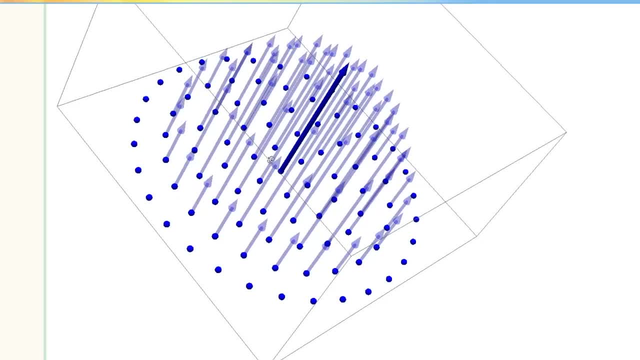 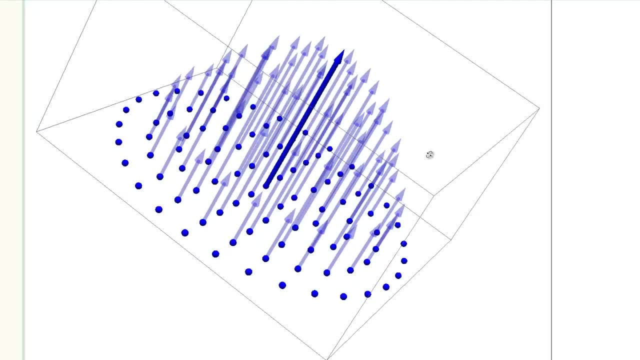 As you can see, on the rim of the pipe you have 0 velocity and towards the center, this dark blue line, here you have the highest velocity. I hope you now understand how fluids flow in pipes and rivers and that you will be. 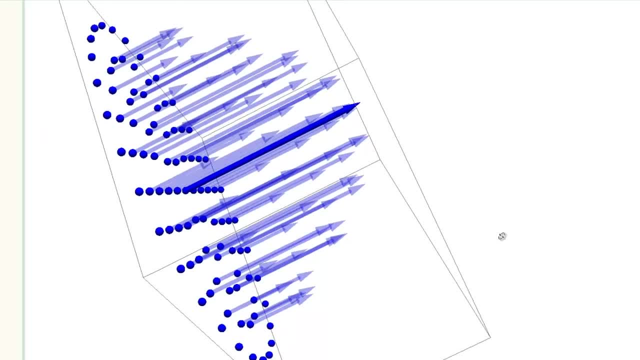 able to apply the Navier-Stokes equations to solve these problems. Thank you for watching.